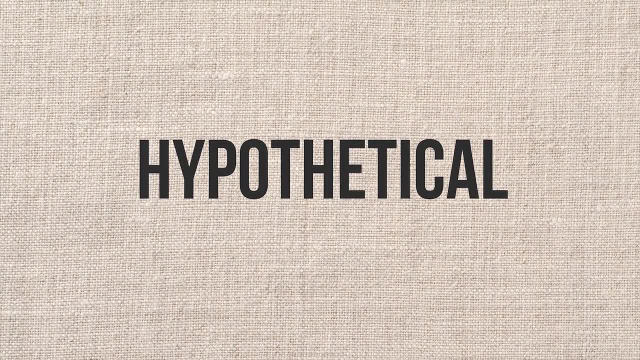 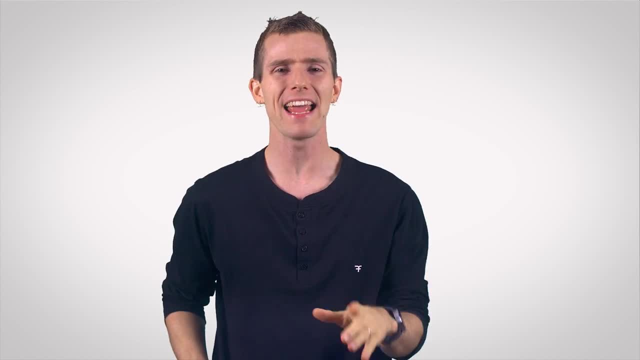 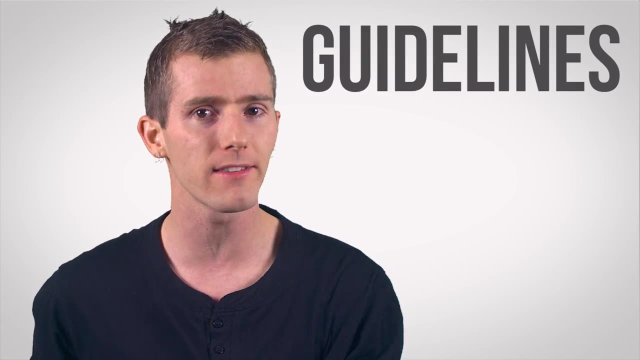 material is more like this hypothetical material out of which all the UI elements, buttons, icons and themes are constructed. And constructed is key here, because material- and I'm gonna keep finger quotes-ing- that must behave according to a number of guidelines set out in Google's material design spec sheet a. 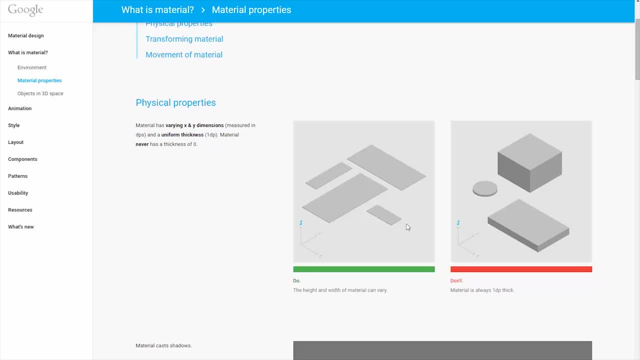 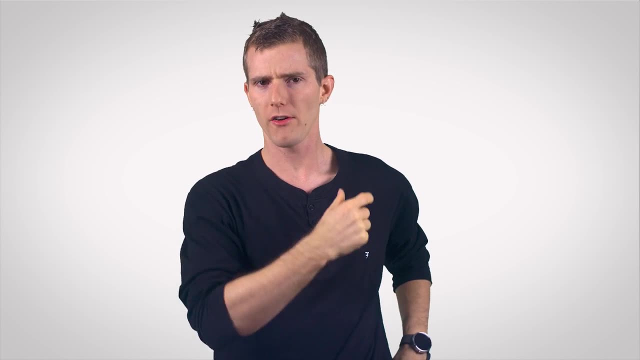 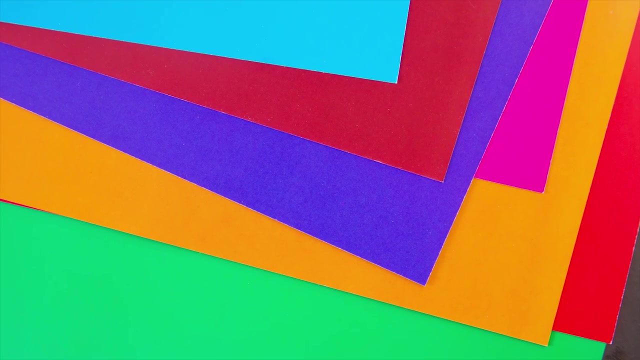 living document that was created to guide artists to make a more unified look for Lollipop and presumably, other Google products in the future. Alright then, Linus. so what are these guidelines? you say? Well, first, much like construction paper, material can come in many different shapes when you look at it head-on. but while it's almost flat, it is. 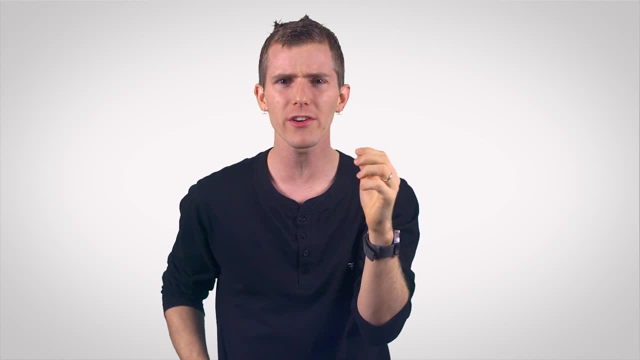 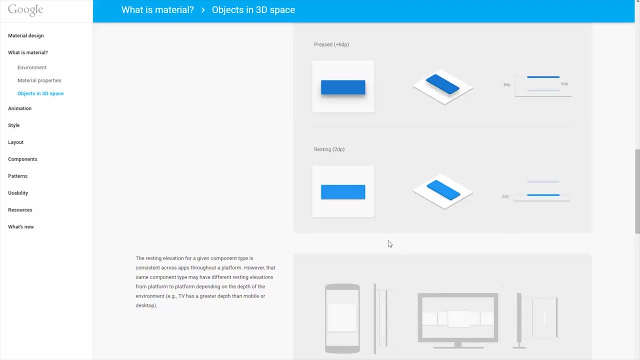 solid, so it does have a little bit of depth to it. All material is exactly one dp thick, even when content is displayed on top of it, which is not the same as one pixel thick, by the way, to allow for a consistent appearance on high. 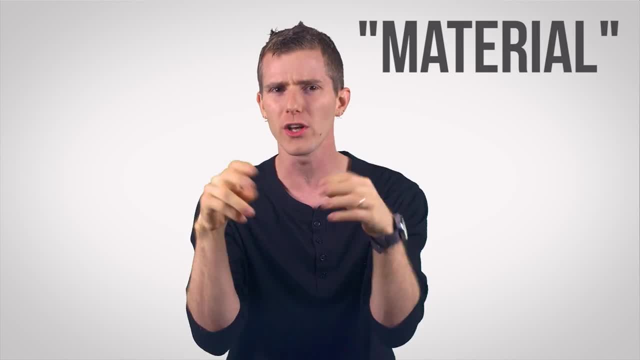 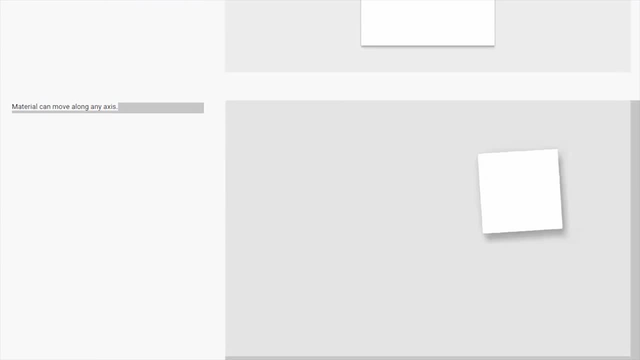 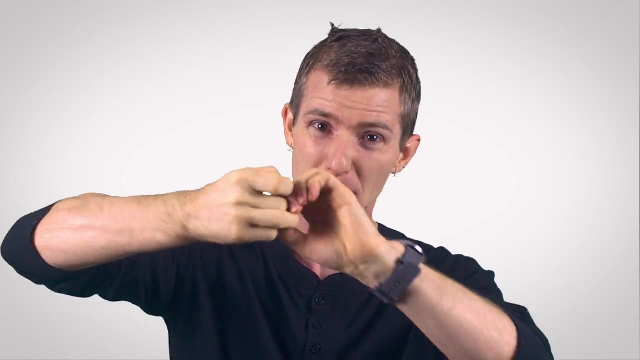 and low resolution displays. Now, because material has that depth, some more rules apply. While it can change shape, grow, shrink and be moved and rotated along any axis, it's solid so you can't click or see through it. Two pieces can't occupy the same space at the same time. 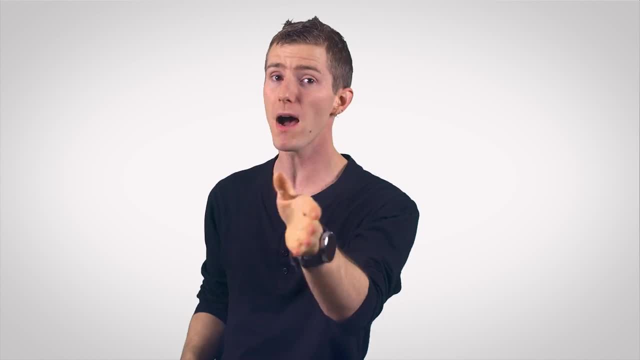 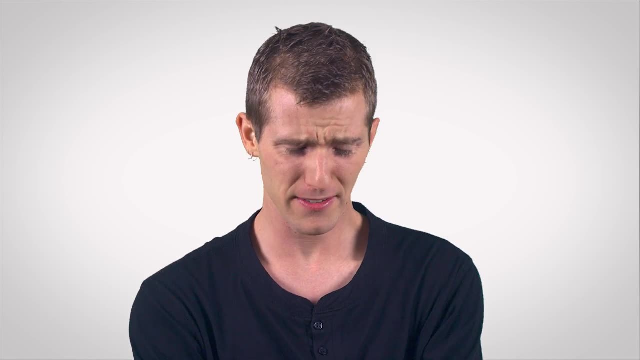 in the same way that my hands can't occupy the same space at the same time, one must be above the other and it can't pass through other material. It also can't bend or fold. Alright, Linus, this is starting to sound like a bunch of arbitrary hipster design crap to me. Why does any of this matter? 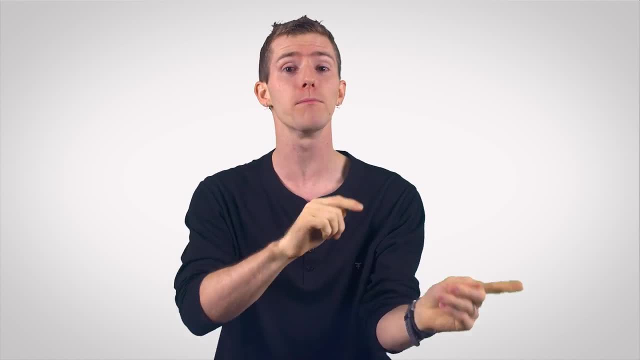 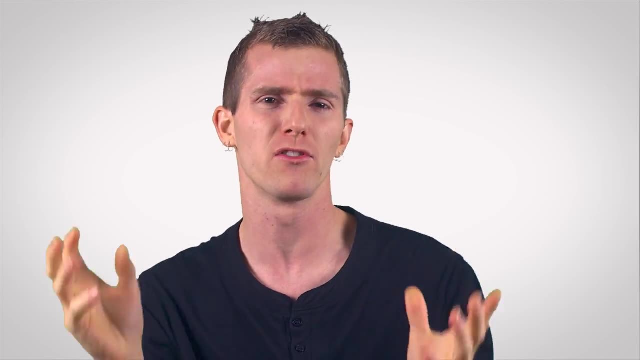 Well, believe it or not, design philosophies like this matter more than you'd think, because material design extends much further than just rules for what app layouts and buttons look like. It's a whole set of guidelines for how we interact with our devices, including things like 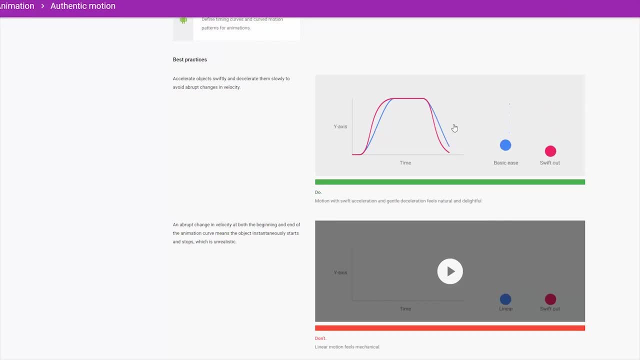 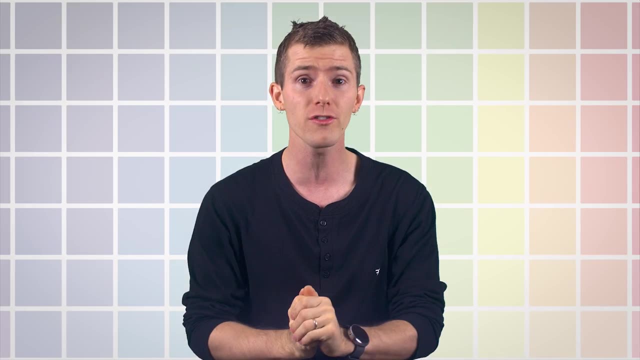 realistic movement animations which, combined with other techniques for drawing the user's eye to the correct part of the screen, enables more natural interaction. There are also color suggestions, so every app on your phone or tablet can have its own unique visual identity, yet be part of a greater. 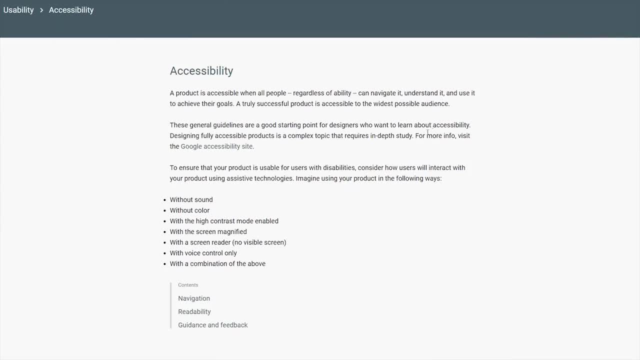 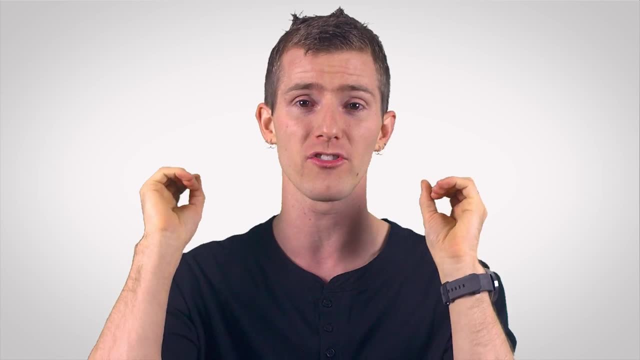 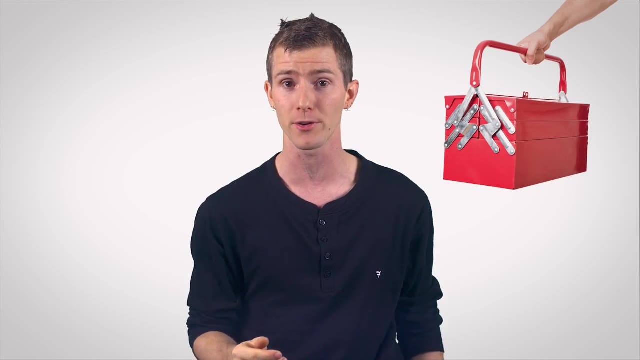 whole, and even advice for developers about how to make sure their product is accessible for users with disabilities. So while I unfortunately cannot stand here and go into as much depth as I could on a topic like this, I hope it was enough to explain the importance of material design as a toolkit for app developers to help.